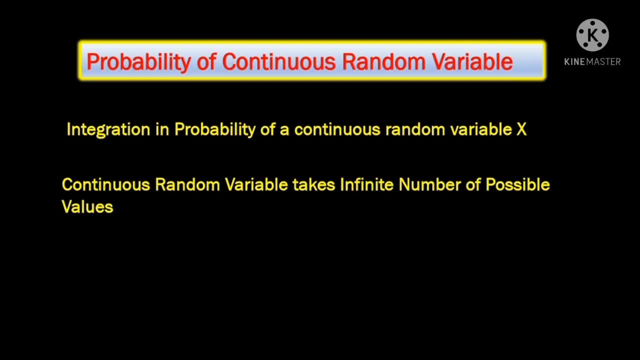 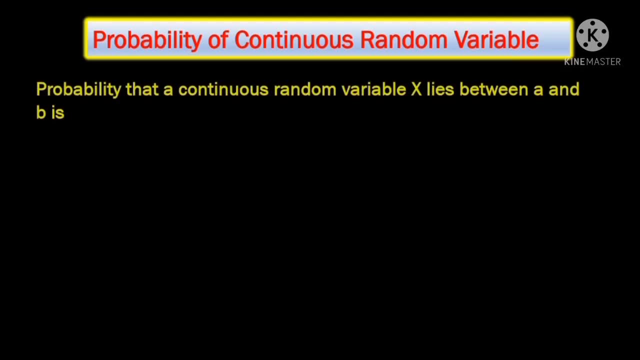 can take infinite number of seconds to find the probability of continuous random variable. So the probability of a continuous random variable x is given by integration a to b, of f, of x, dx. So, friends, how does integration come into the picture? Well, that's because the area 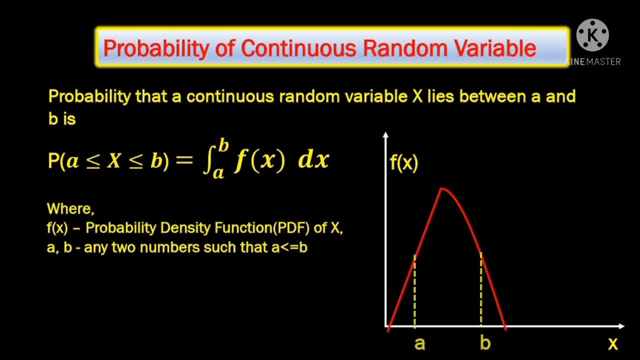 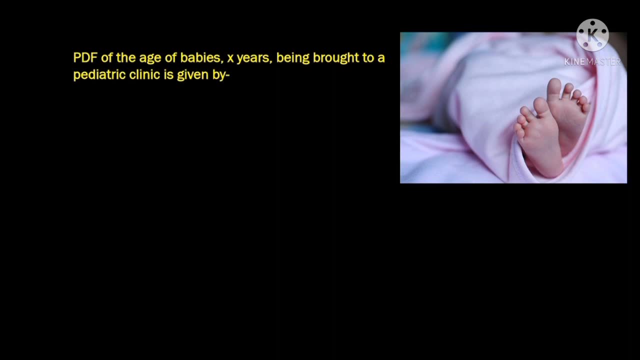 under the curve of f of x and x from a to b always gives you the probability which can be very easily found by integrating the given function from 0 to 2 by 3.. So, friends, let's apply this to a pediatric clinic, where the probability function of age of babies is given by this equation. Now, 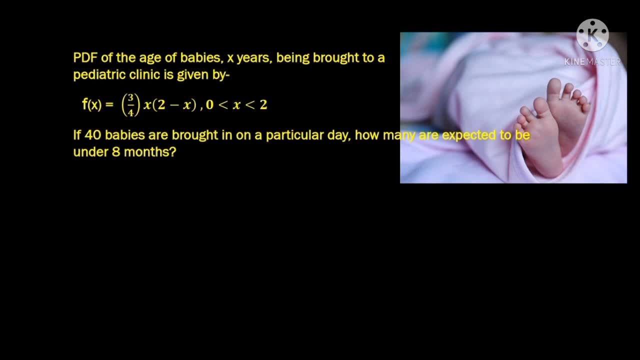 if around 40 babies are brought on a particular day, how many can we expect to be under 8 months? So this probability can be easily found by integrating the given function from 0 to 2 by 3 and friends. by doing these calculations we can arrive at the conclusion. 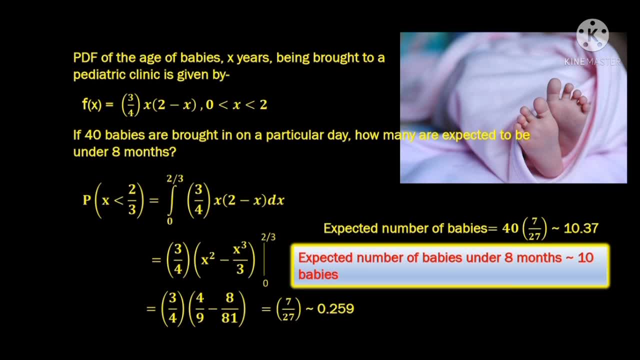 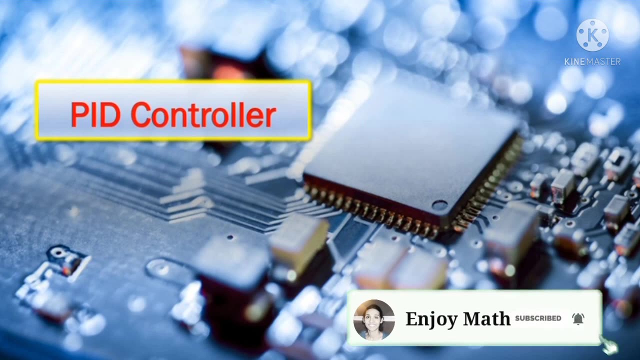 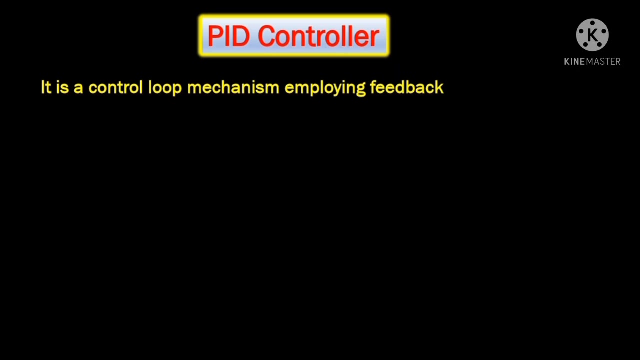 that the expected number of babies under 8 months is approximately 10.. So probability of continuous random variables without integration is indeed hard to imagine. Let's now see how integration plays a very important role in PID controller. So the PID controller is nothing but a control loop mechanism with feedback and friends. 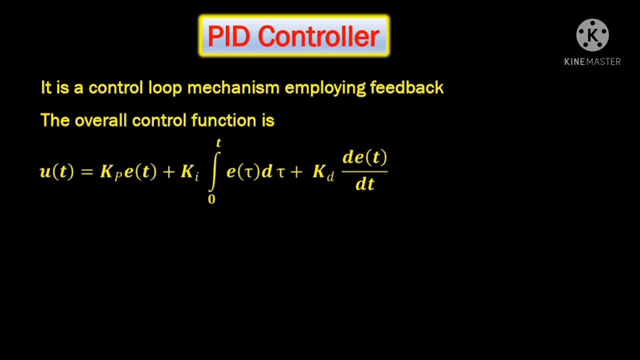 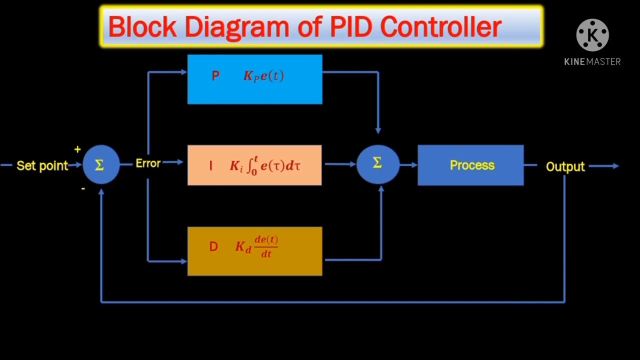 here is the overall control function, where Kp, Ki and Kd are the coefficients for proportional integral and the derivative terms. Now the PID controller continuously calculates an error value and this integral unit measures the area between the error values and helps the system to tune into an error of 0.. 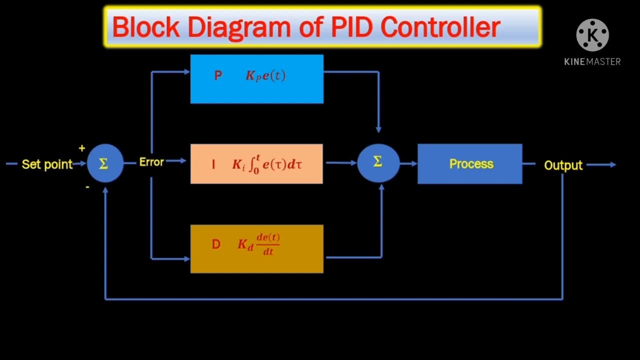 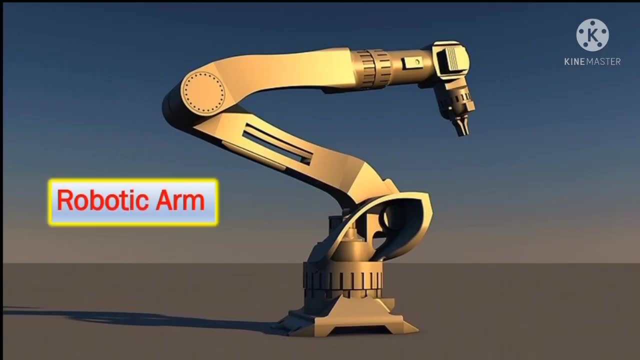 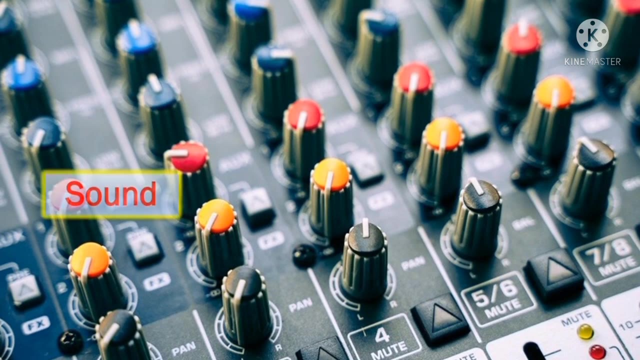 Now, friends, this PID controller is extensively used in many fields, including the car cruise control, which is so widely used, and also in the movement and of a robotic arm. friends, let's now see how integration is so powerful in the world of sounds. now, the sound power passing through an area can be easily. 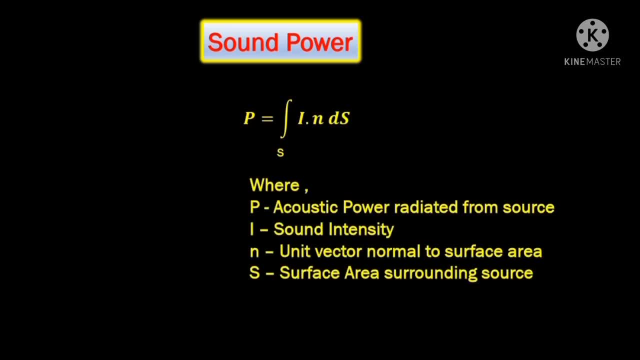 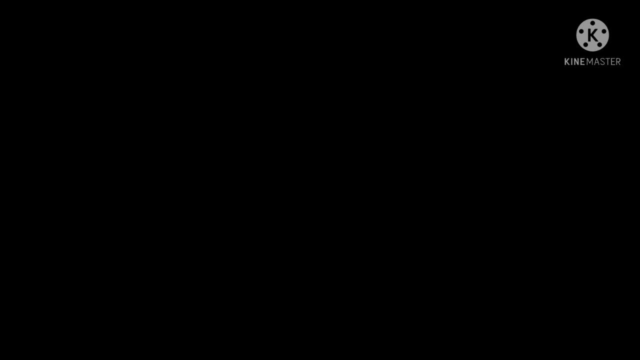 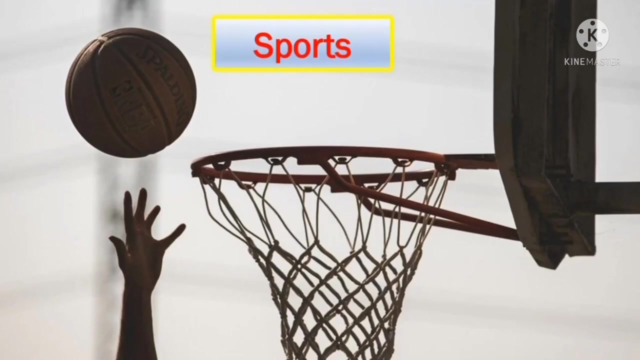 obtained by integrating the sound intensity over an imaginary surface surrounding the source. now, friends, this sound power is very important because it helps predict the sound impact of musical performance venues. we can easily decide if the music is too powerful, like this, or if it's too weak for the audience to enjoy. like this, friends are surprising. 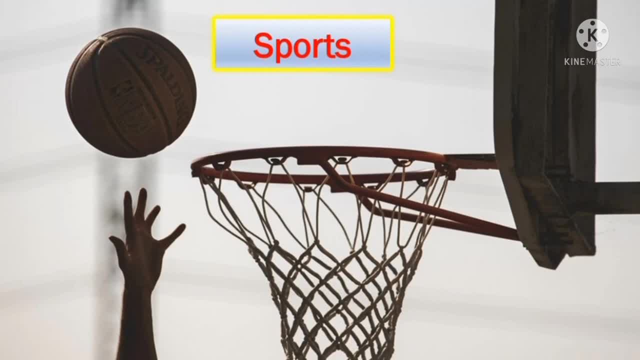 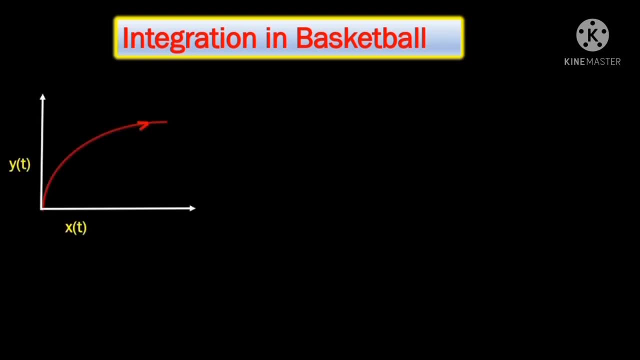 but true that integration helps analyze sports better. let's see how you. let's consider basketball, in which we need to find the length of the arc that is formed by the ball. so, friends, here we need integration because the arc length formula is the definite integral of the velocity function and time. so, friends, if 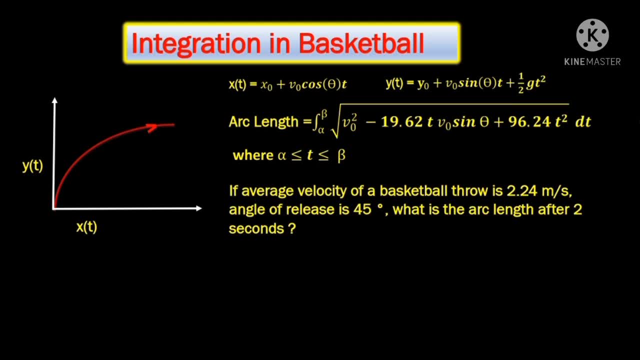 the velocity of the ball is 2.24 meters per second at an angle of 45 degrees, then the arc length, say after 2 seconds, can be found by putting these values in the formula to get the arc length to be 17.34 meters. 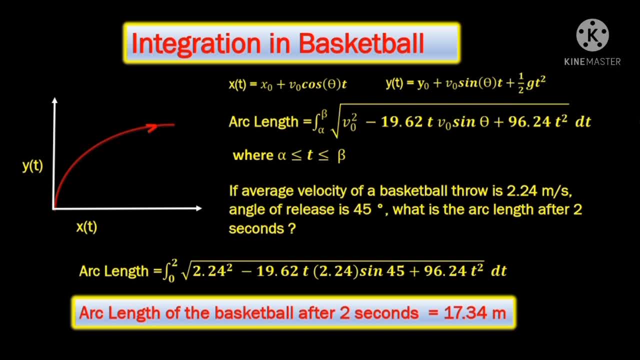 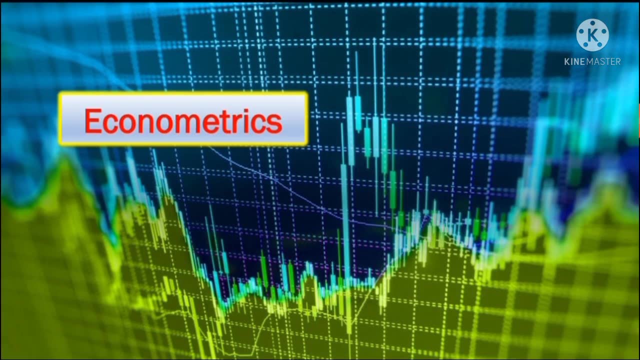 and friends. in this way, integration helps in giving important game related statistics to improve the team and the player performances. let's now see how important integration is in econometrics. so, friends, here is the Lawrence curve which graphically represents the inequality involved, or any other system. it plots the cumulative income in the 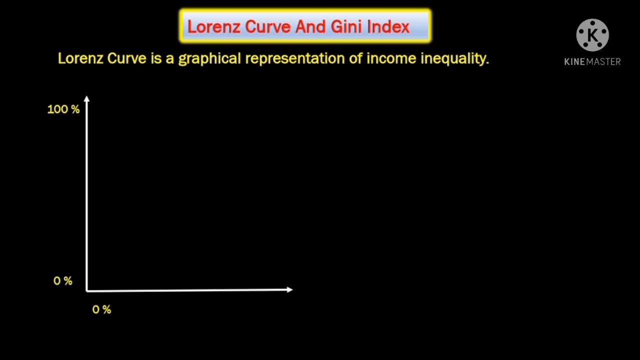 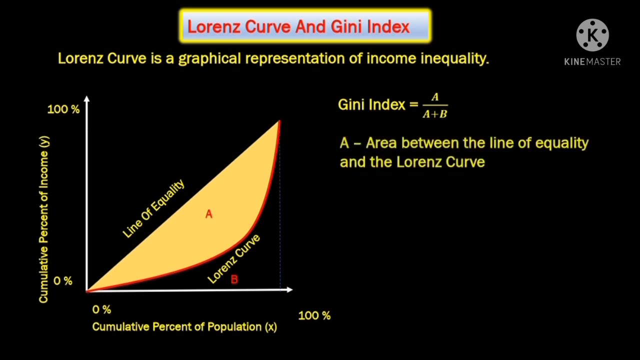 system 제 aguinne engraving ny om. I am a against cumulative population. Now we can measure this inequality using a very useful index called the Gini index. It is calculated as the ratio of the area between the perfect equality line and the Lorentz curve to the total area under the equality line. And friends, because we have 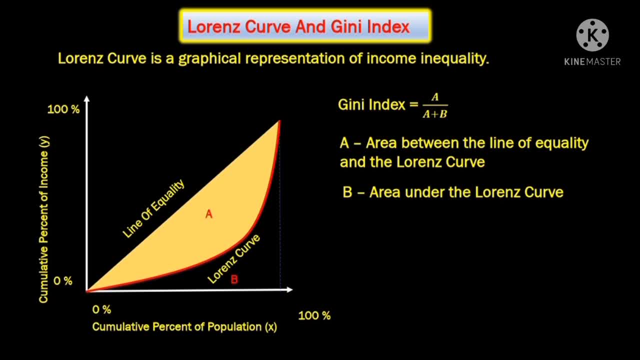 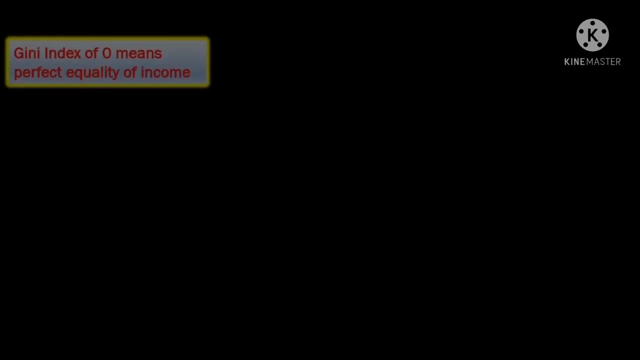 area under graph, integration definitely comes into play and the Gini index is given by this integration formula. So by calculating the Gini index of a country we can determine how the wealth is distributed. So if the area under the graph is 0, it represents perfect equality of income with 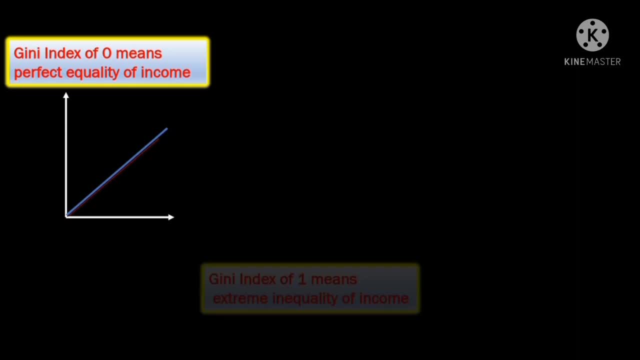 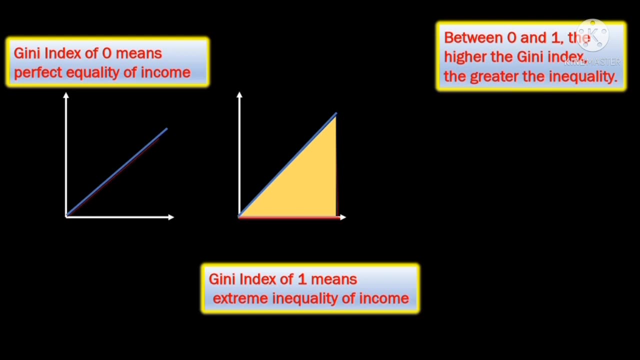 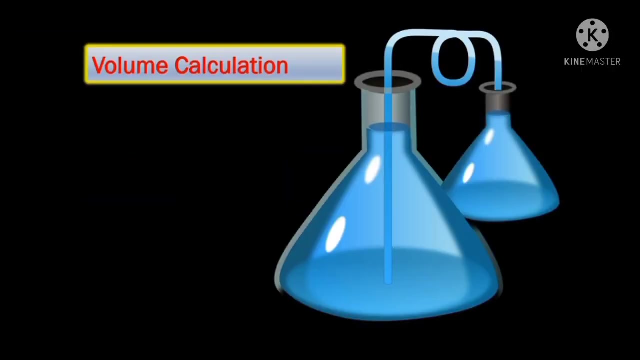 0 Gini index. On the other hand, the Gini index of 1 shows extreme inequality in the income. The value of this index hovers between 0 and 1, and the higher the Gini index, the greater the inequality. So integration is indeed very useful in econometrics Friends. integration is also very useful to 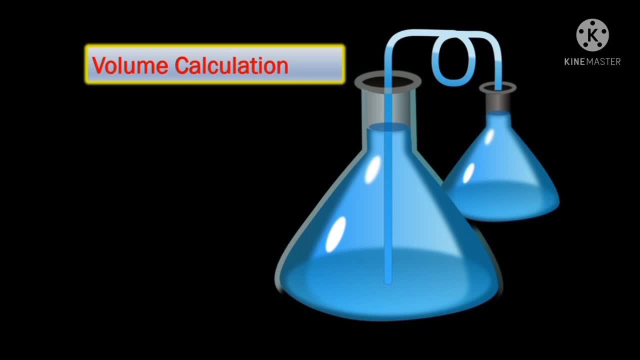 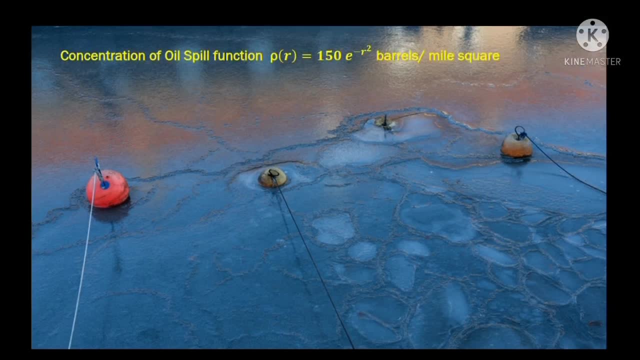 calculate the volumes of different regions. Let's see how, with this example of an ocean oil spill, the concentration of the oil is given by this function. Now, if the spill has reached a maximum radius of 5 miles, let's calculate how much oil was spilled. So, friends, this 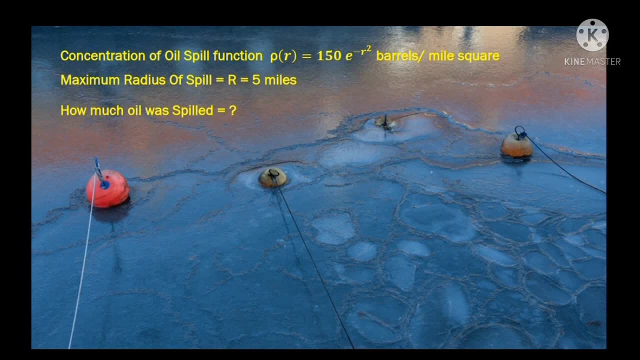 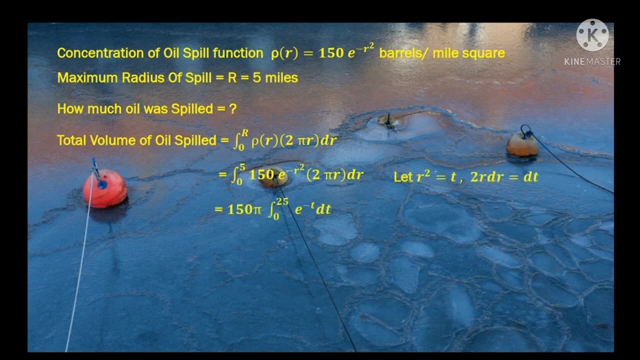 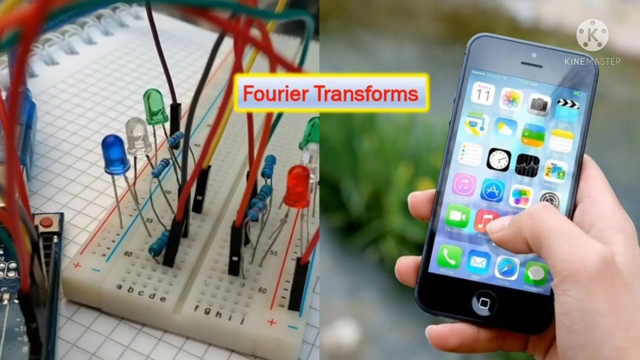 region of the oil spill can be found using the disc method of integration to arrive at this formula. and, friends, by substituting the different values, we can conclude that the total volume of oil that is spilled is 471.428 barrels. And friends, last but not the least, let's see how. 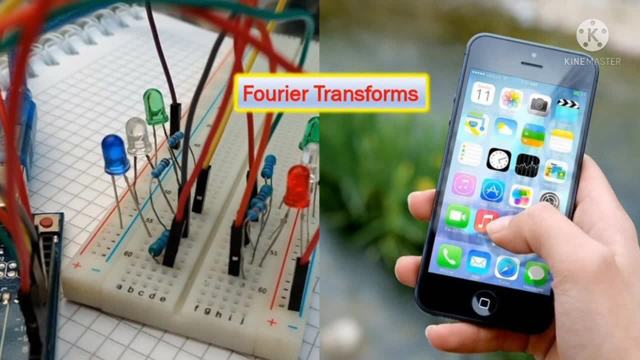 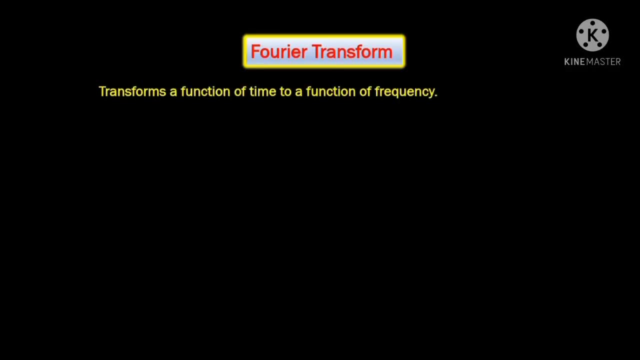 integration in Fourier transforms is helping transform the world. So the Fourier transforms simply changes a function of time to a function of frequency and friends. here is the main integration equation that relates the function of time and the function of frequency. Now Fourier transforms is used extensively in finding 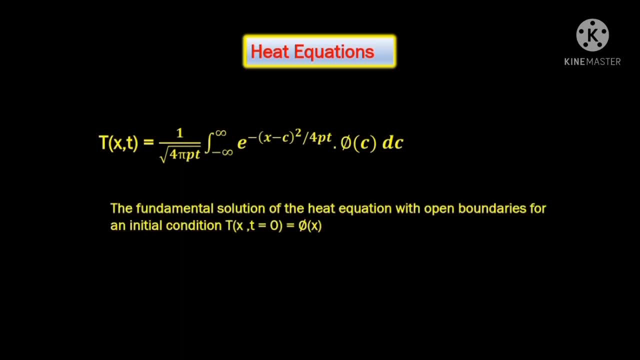 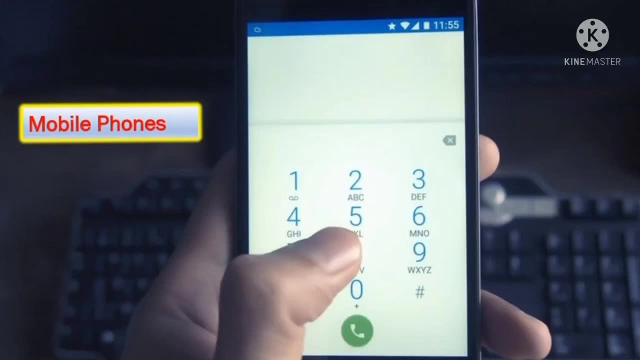 solutions of heat flow equations. It is also used in analysis of electrical circuits and also processing different signals And friends. It's also used in all mobile phones when you are punching in the numbers. As Fourier transform of these input numbers are done for further processing. 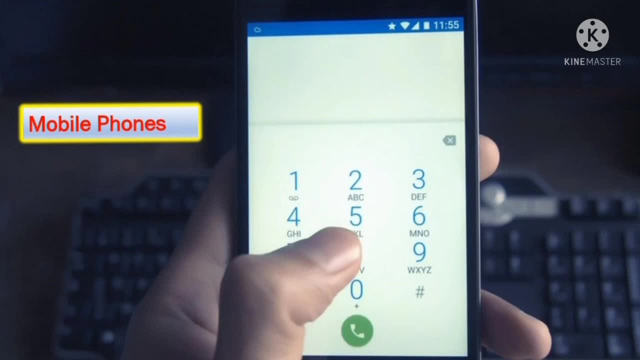 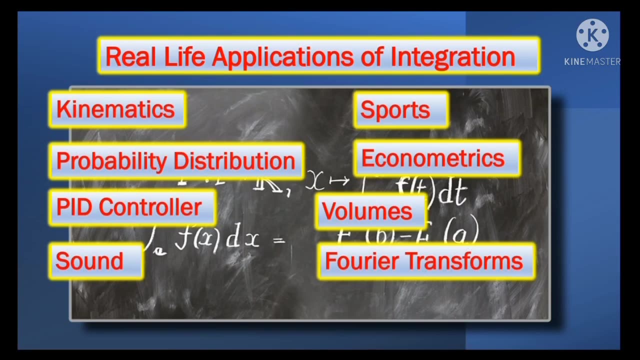 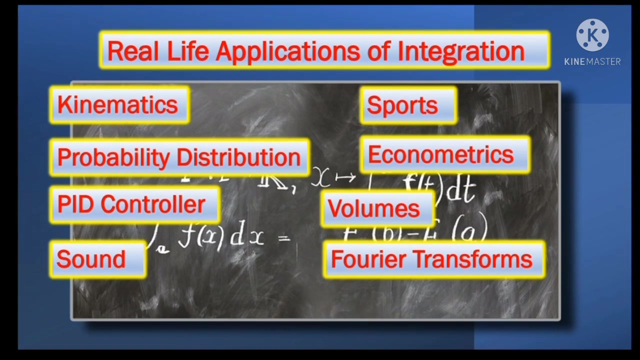 So integration in Fourier transforms is invaluable in today's world. So, friends, to summarize this video, here are the applications that we have discussed. and, friends, these are just some of the numerous applications of integration. So, friends, if you found this video useful, do like and share. please do leave your comments. 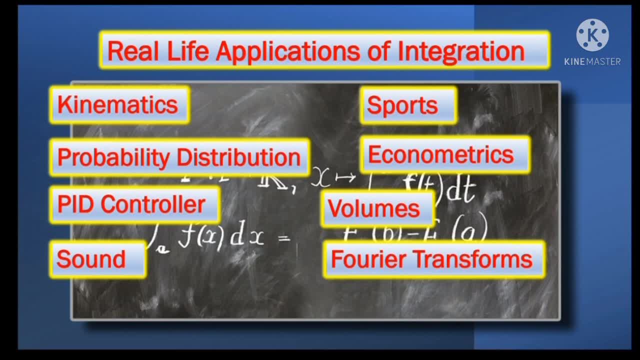 in the comment section below and consider subscribing to enjoy math. So till we meet again in the next video, take care. bye.